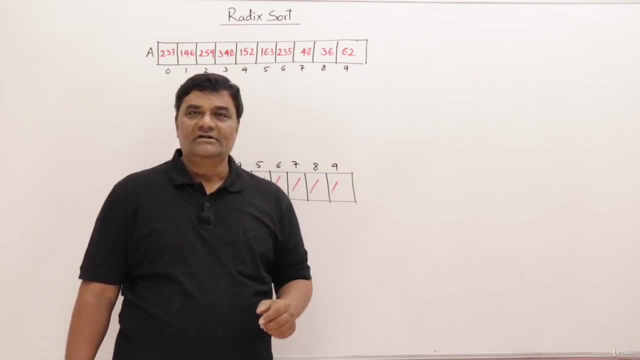 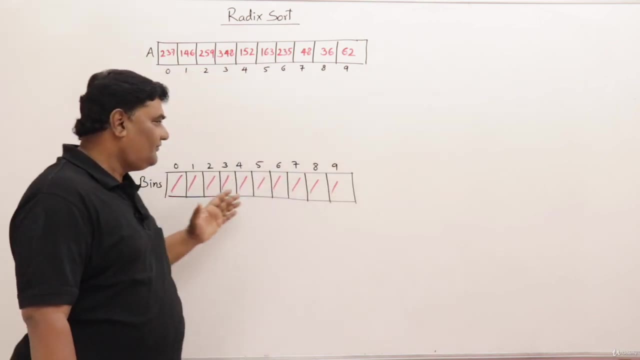 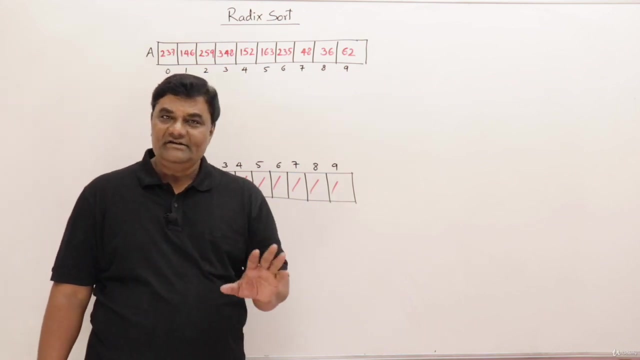 If they are octal, then only 8 bins are enough, 0 to 7.. So that's why the name comes radix sort. So for sorting this decimal numbers I have already taken 10 bins and also initialize them to null. So setup is ready. Next we have to learn how to sort them. So let us start sorting the numbers. So let us start the procedure. In the procedure I will scan through: 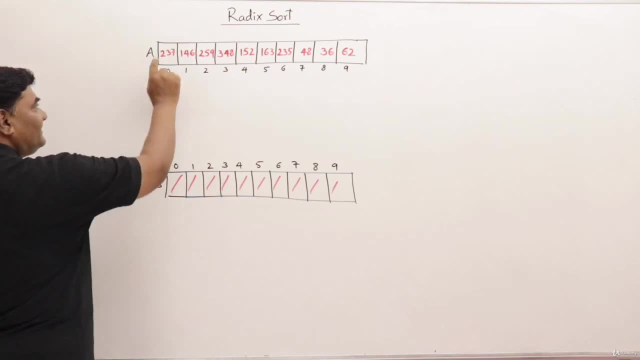 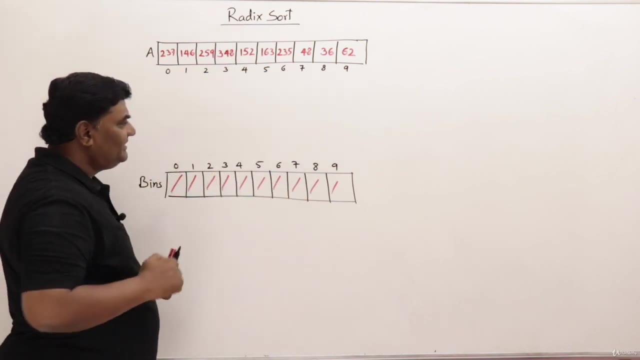 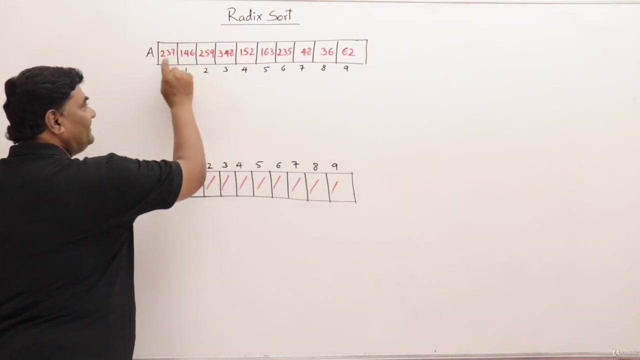 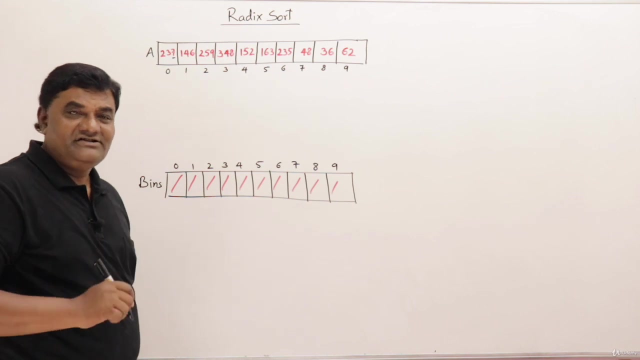 this list of elements And every element: example 237.. For 237, there is no bin available here. No, no, you don't have to drop it in bin 237. You have to drop it in bin 7.. So it means I should just check last digit of a number. Yes, just check last digit and drop it in that corresponding bin. So this is 237 will get dropped. 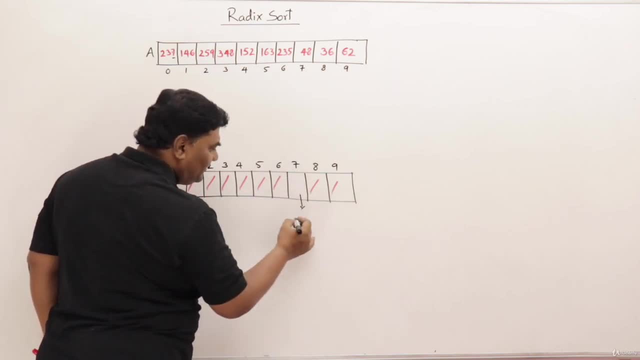 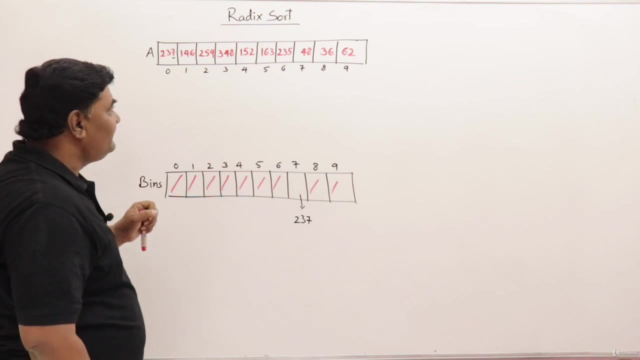 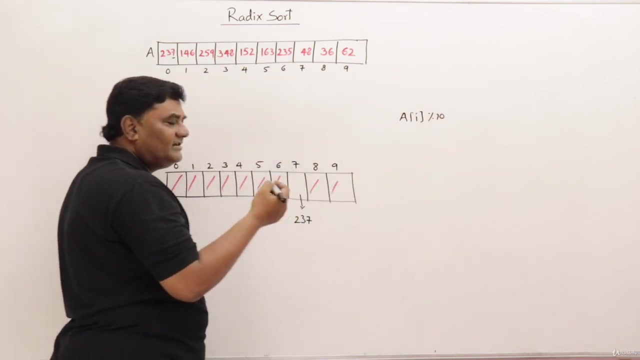 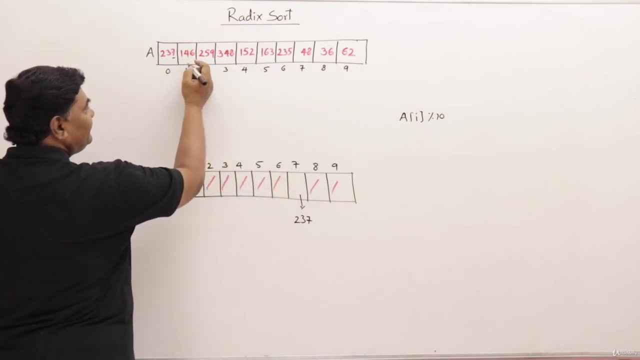 Here in the bin 7.. So I will not draw nodes and all, I will just write number 237.. It is dropped here. So how I can know that last digit? So, whatever the number is, if it is a of, i then mod it by 10, you get the number. So, last digit, you will get. Yes. Now, same thing, I will do it for all: 146.. This is 6.. It will go into bin 6.. 146. 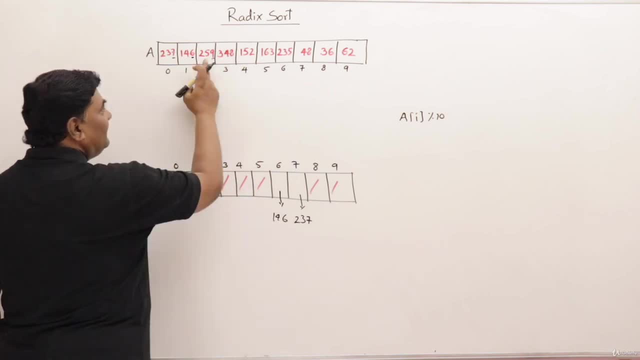 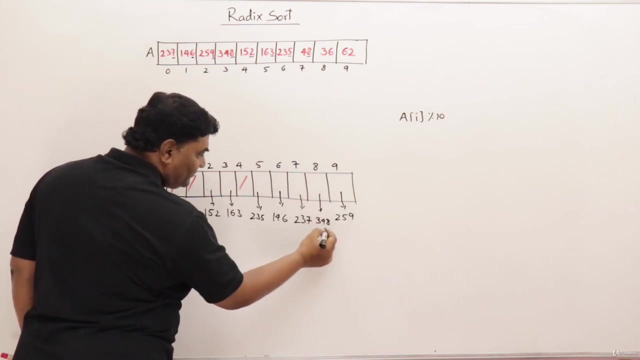 The next is 259.. It will go to bin 9.. 259.. Next is 348.. Bin 8. 152.. Bin 2. 163.. Bin 3. 235.. Bin 5. 48. Bin 8. Already number is there, So below that, 48. 36. Bin 6. Already number is there. 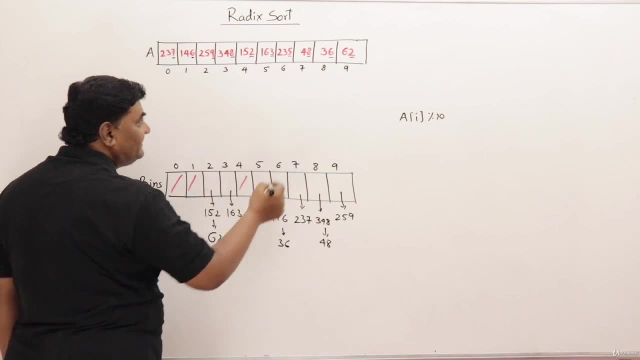 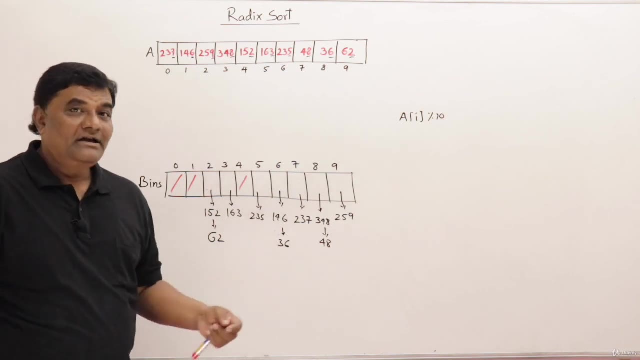 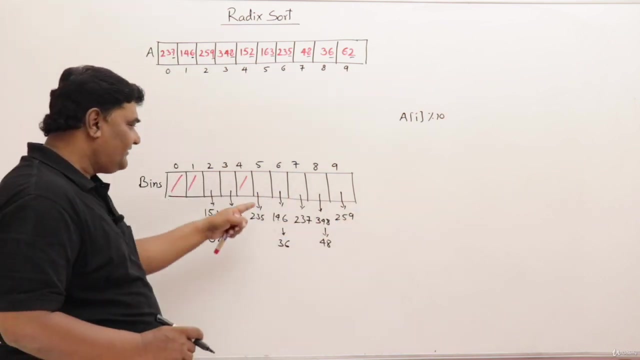 So below that, 36.. So 62 is here in bin 2.. So all the numbers I have scanned and I have filled them in their corresponding bins based on the last digit. Are they sorted? Let us see. I have to take out all these elements from all the bins, one by one, by scanning through all these bins Right, One by one, take out all the elements. As I said, these are FIFO. Don't go like a stack, Don't follow LIFO, Follow FIFO. 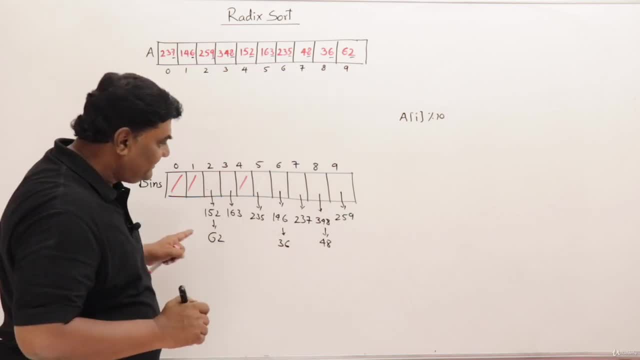 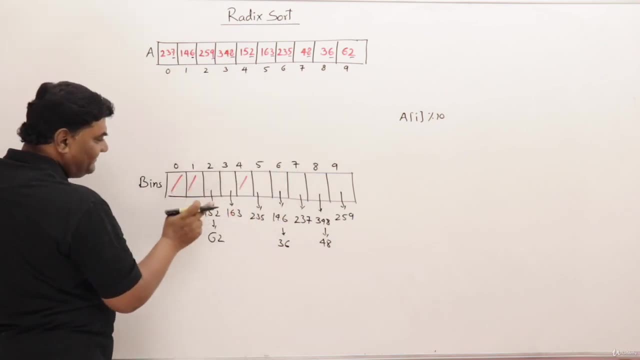 First element: take it out first. The next element: take it out next. So let us follow the order. I will be emptying bins and I will write down the elements here. So let us start. This bin is empty. This bin is empty. This is 152.. So write down 152.. The next is 62.. 62.. I will separate them by comma, So these elements are gone. Next is 163.. Next is 235. 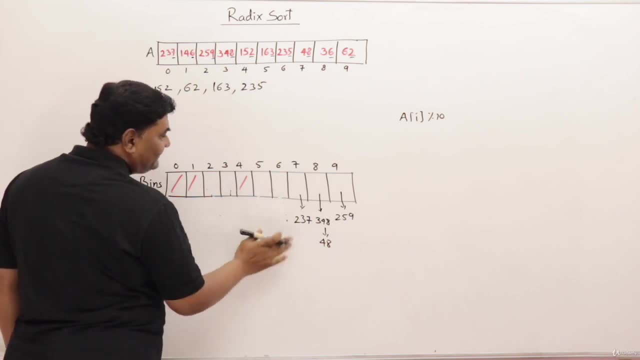 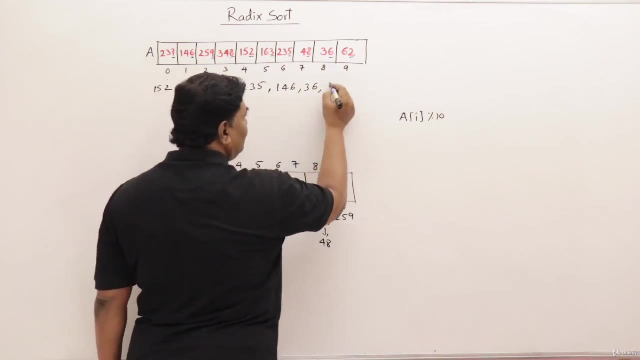 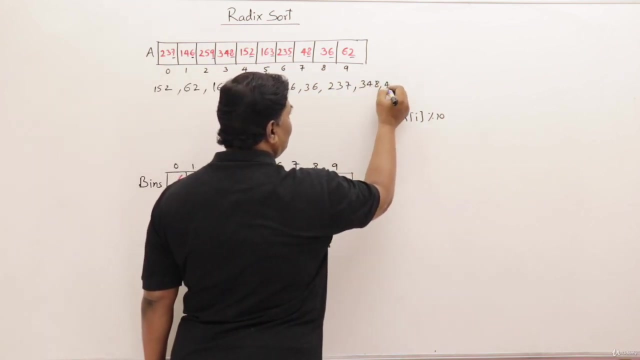 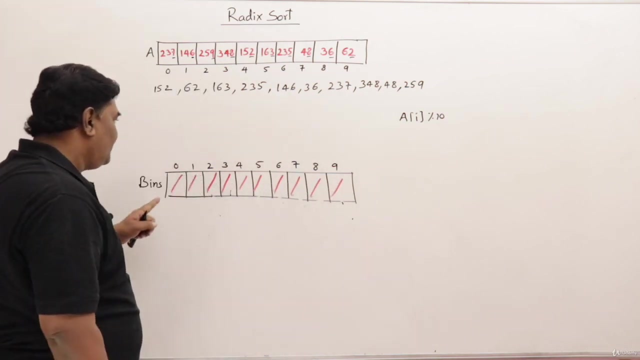 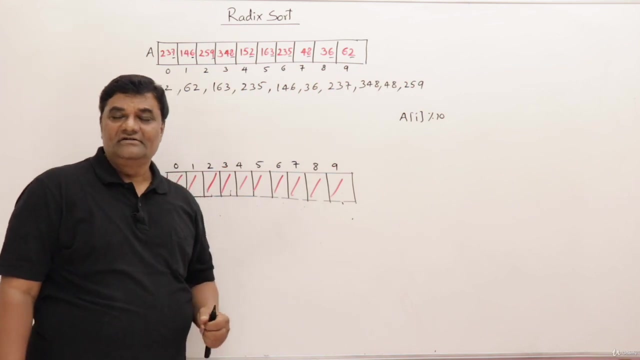 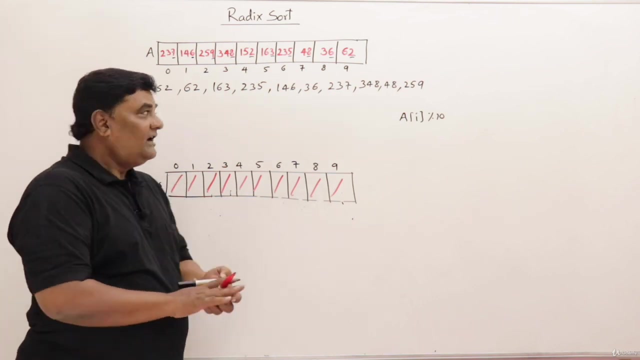 146 and 36.. 237.. 348 and 48.. 259.. So I have emptied all the bins Right And also I made them null. The elements are here. Are they sorted? No, Which is the smallest element, 36.. That should come in the beginning. They are not sorted. They are not sorted Then what? Again, drop them in bins. On what basis? On the second digit from right hand side, Second digit First. we have dropped them based on this last digit Now, second digit from right hand side. 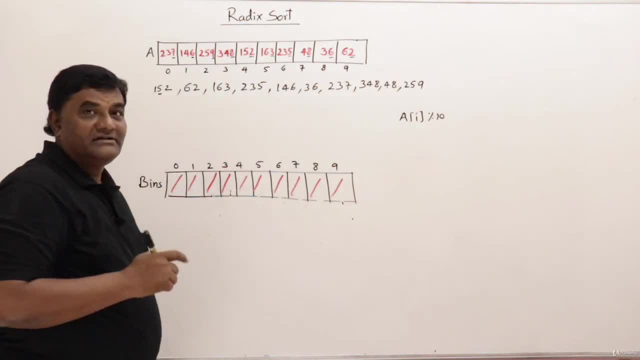 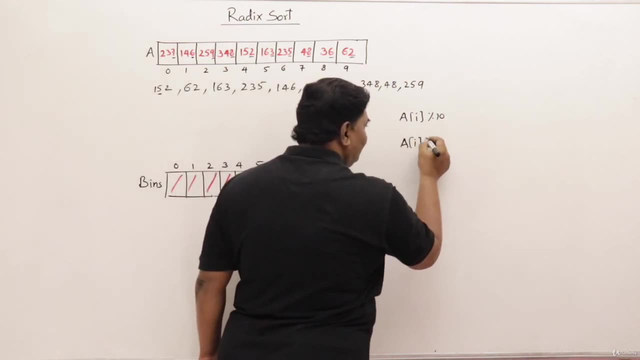 Second last digit, or second digit from right hand side, Second digit: How to take out that second digit? So, for any element, what I should do is divide it by 10.. So if I divide it by 10,, like 152,, if I divide it by 10, then I get 15.. Then mod by 10.. Okay, if I mod by 10, then I get 5.. Yes, So divide by 10 and mod by 10.. 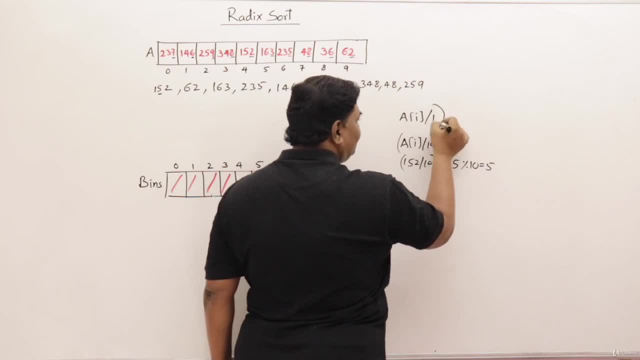 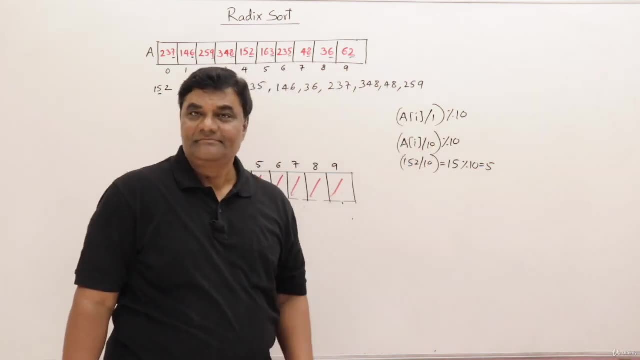 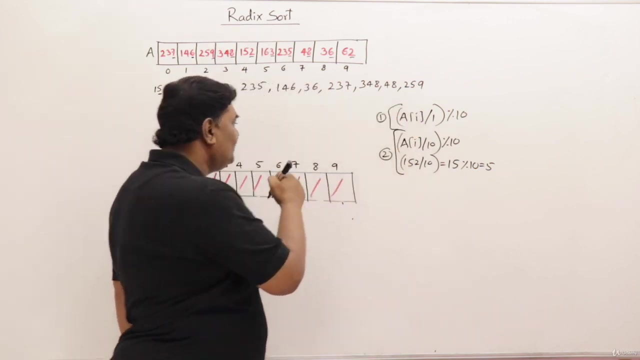 So that means earlier what we did: Divide by 1 and then mod by 10.. That's what we did. Now that division number has become 10 next time. Okay, we will follow this now. Right, This was the first time we have done and this is the second time we will do that. So first pass is completed and this is the result of the first pass. 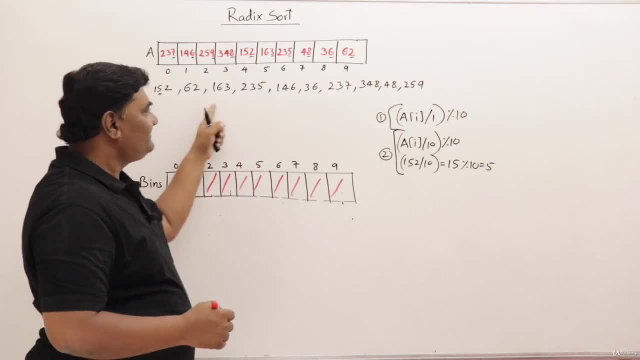 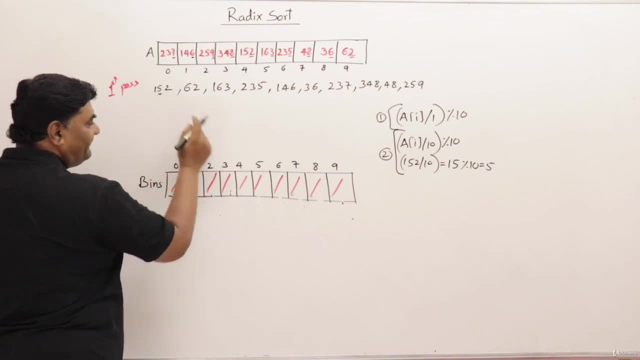 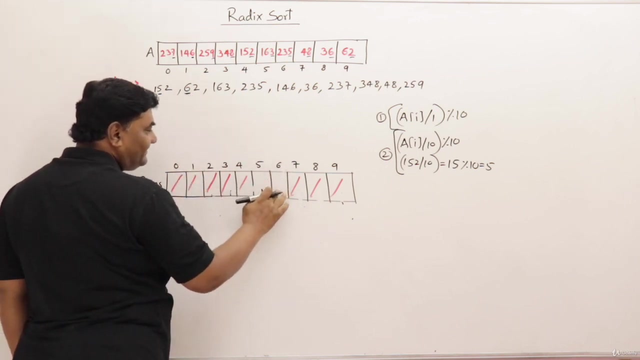 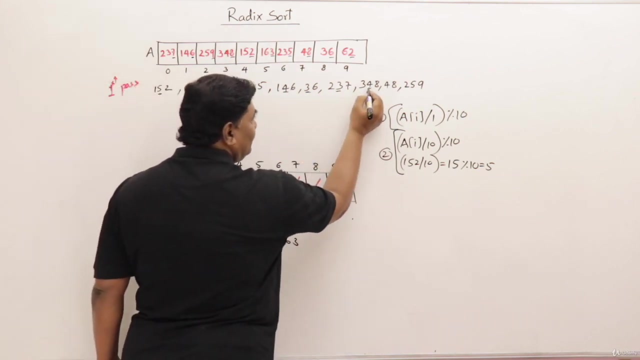 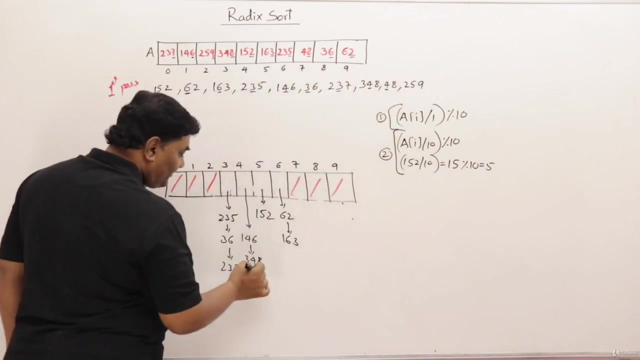 Okay, The second pass. So let me do it now: 36 bin 3, 237 bin 3, 348 bin 4, 48 bin 4, 259 bin 5.. So I have dropped all those elements once again from array A into bin. 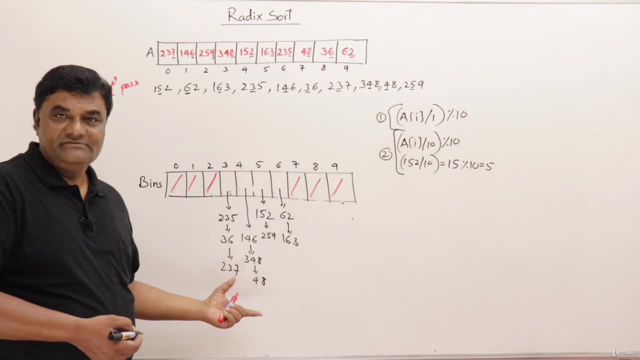 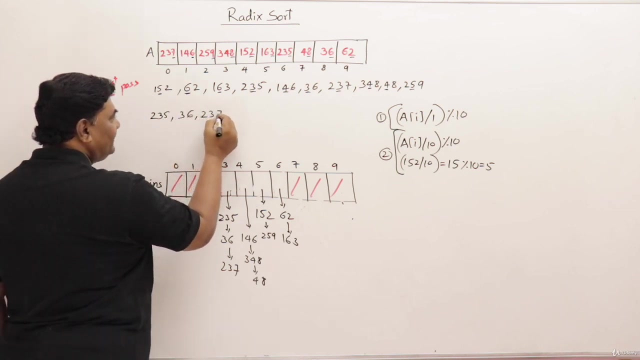 Now empty all these bins one by one. So I will write the result here: Empty, empty, empty. 235, 36, 237.. 235, 36, 237.. So these are all gone: 146, 348, 48.. 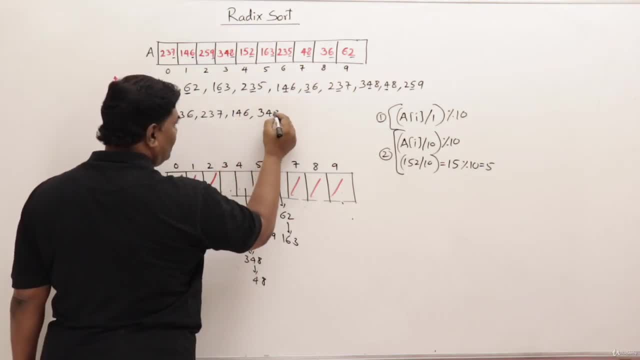 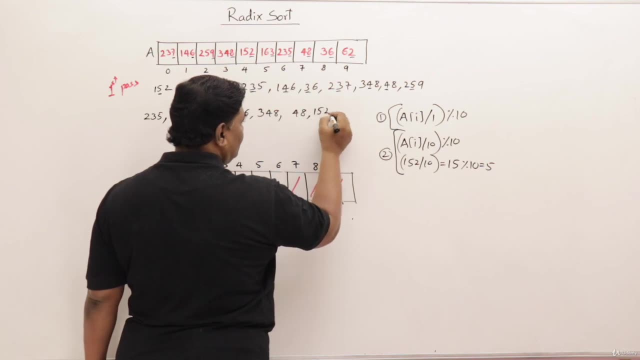 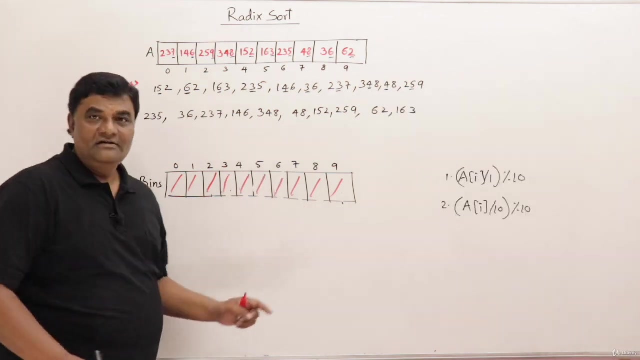 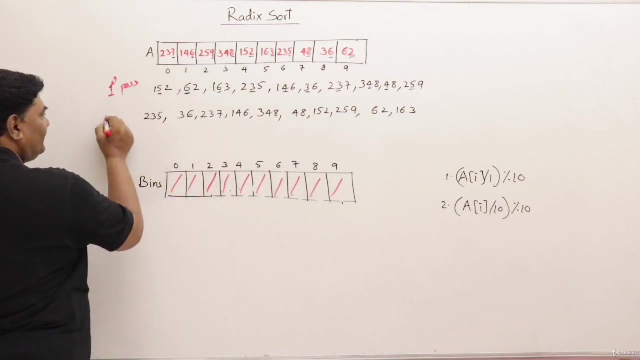 48., 152,, 259., 62 and 163.. So I have emptied all these bins and the elements are written here. So this is the result of the second pass. So I did two passes over. Check: are the elements sorted? 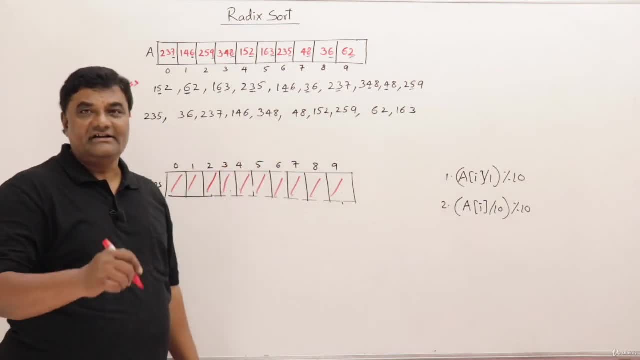 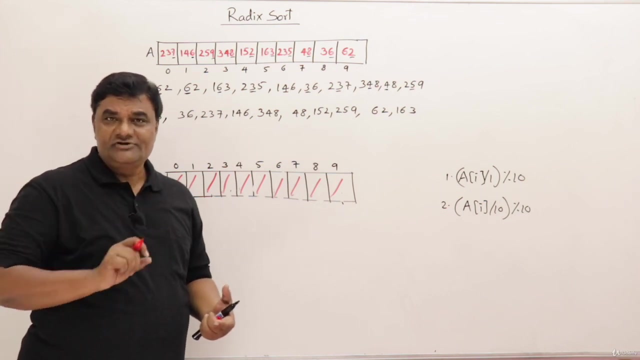 Smallest element is 36.. That should come first. It's not there. They are not sorted. Then what Repeat for one more pass, One more time? you do it Already two times we have done. Why third time, We did not get them sorted? 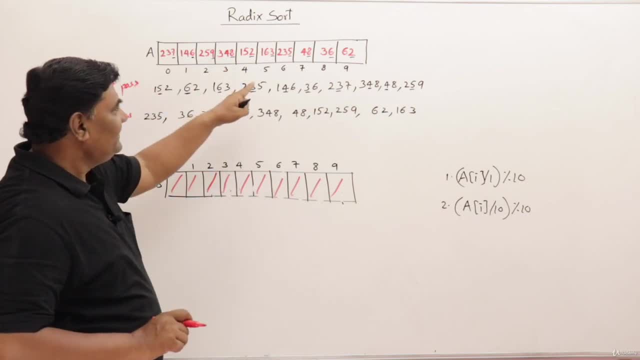 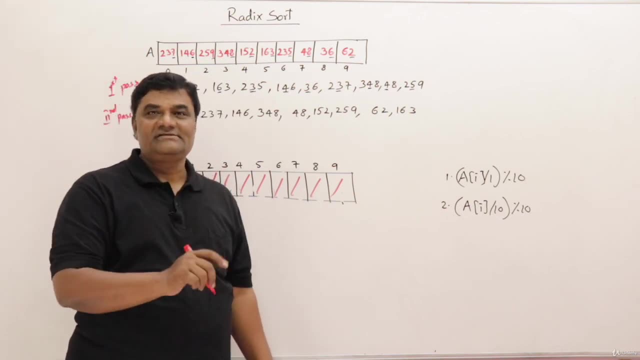 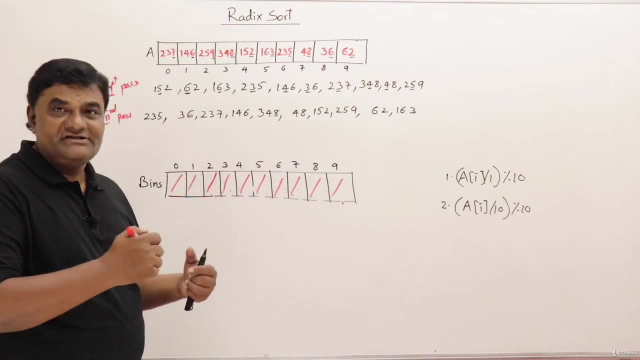 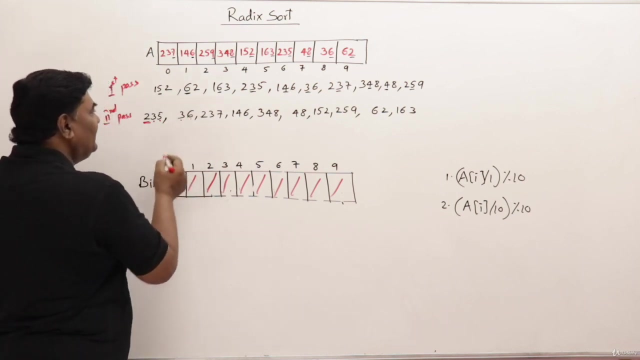 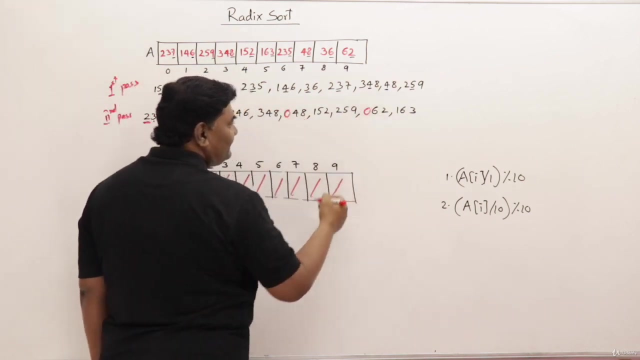 Yes, Then see the digits. if you see, The largest number, that is 348, is of a three digit. So you have to perform three passes. After three passes they will get sorted. Okay, Let us try it for one more pass now, based on which digit we should do. we have finished upon rightmost digit, then the second digit also. now we will do it on third digit. so it means first digit from right side it is third digit. what about this? two digits only. then assume this digit is zero. okay, so for 48, also, this digit is zero. 62 also, this digit is zero. so now we will perform upon this one. so how to get this one from this one? 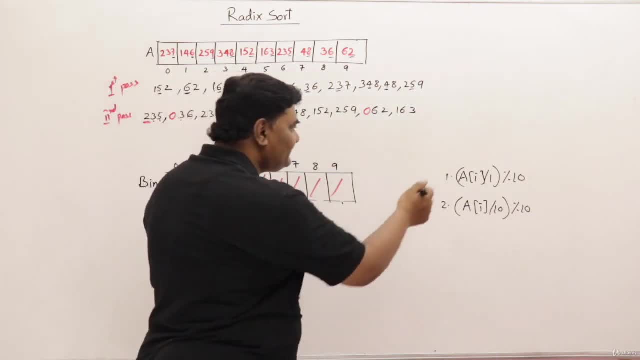 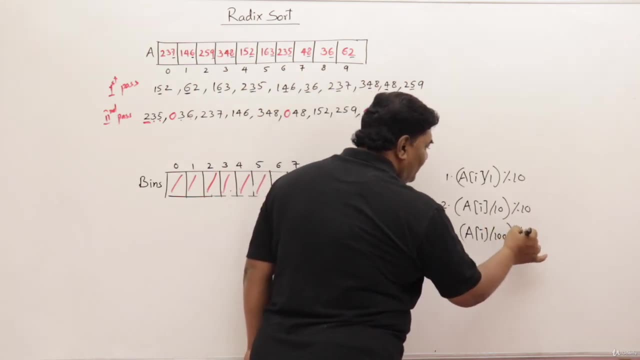 Okay, From 235. how to get two? see similar now in the third pass what I should do. a of I divided by 100 then mod 10. how 235. if I take divided by 100, this gives what result? 2 then mod 10. if I do mod 10 gives answer 2 only. so yes, divide by 100 and mod 2, then you will get third digit. 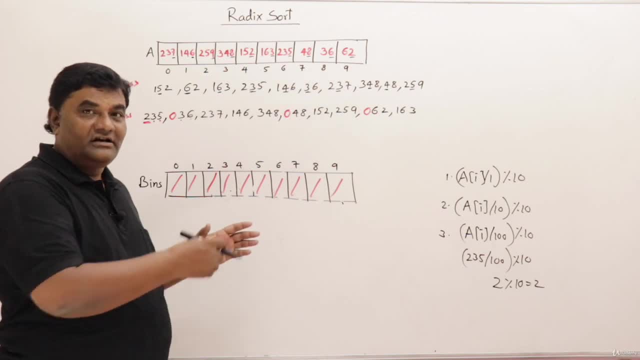 Did you it from the right hand side? Now, based on the third digits on the right side, that is third place. Drop the animals in Venice: 5. do it now. Mod 10 will do. if you guys were the one of the winners, because then one or one, but we get that one. Here once again. Could always take that kind of m Rep. Okay, Mod 10, Yes, This is to. so you should go ahead and go beyond the door so close it by 4 to 35 UH room and side. This isy, but then you know, sort of washer if you were that person are always like, so I always was sorry if I was there. 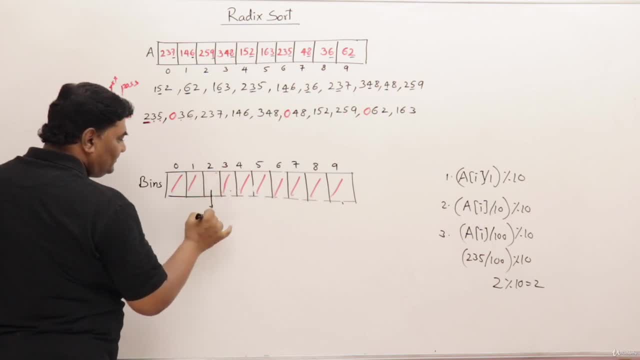 You cannot talk about this fry now, Lab diver. So we're looking at the. got a secret. they should in your shoes as one. So I don't have nothing else more at 0 and to M, please gotta goRE畫hterizi. 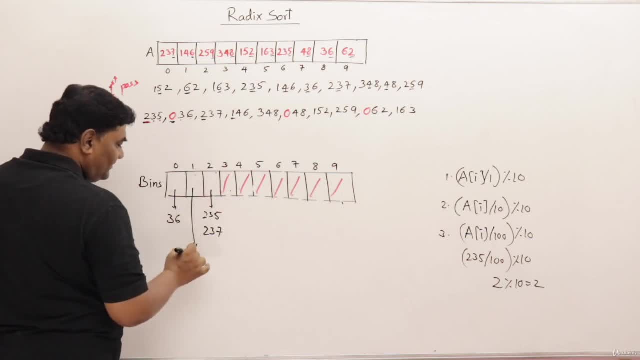 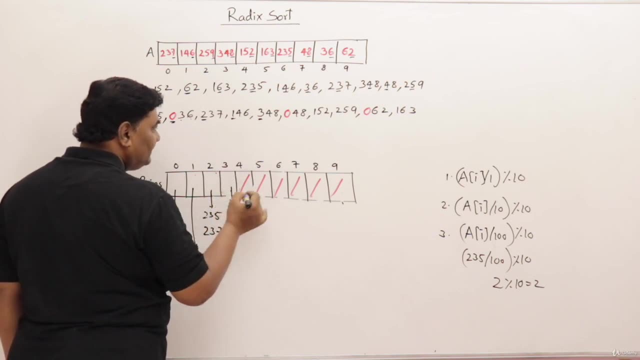 146,. it should go into bin 1.. 146.. 348,. it should go to bin 3.. 348.. Bin 0, 48.. So this is 48.. Bin 1, 152.. Bin 1, 152.. Bin 2, 259.. Bin 2, 259.. 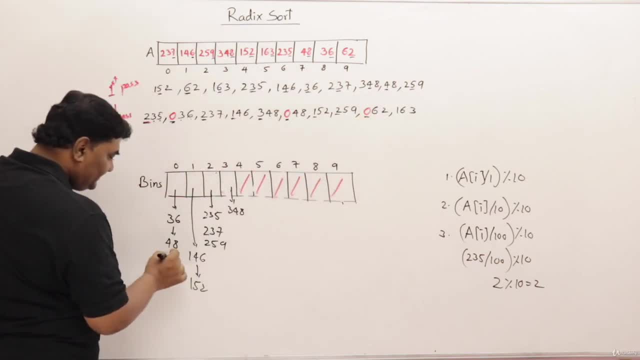 Bin 0, 62.. Bin 0, 62.. Bin 1, 163.. Bin 1, 163.. All elements are completed. Now I should empty all these things. Let us start from first. bin 36, 48, 62.. 36, 48, 62.. Next bin. 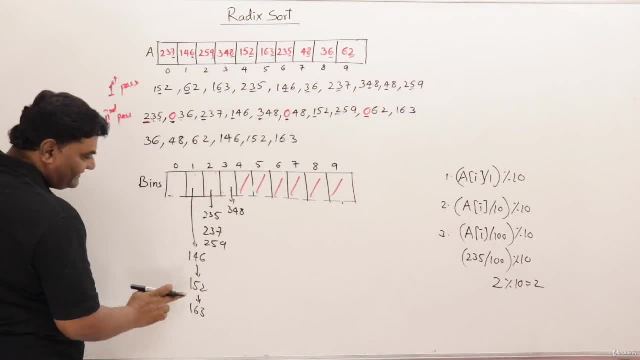 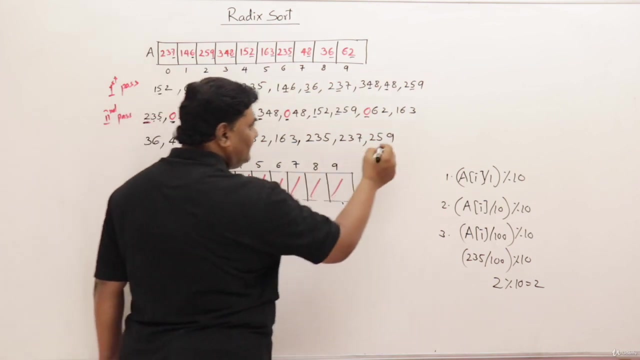 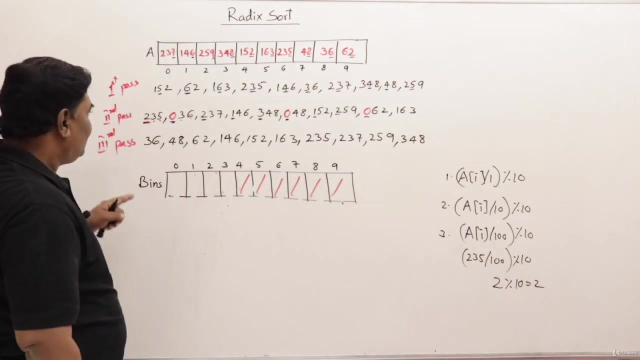 146, 152, 163.. So 146, 152, 163.. 146, 152, 163.. So these are also gone. Next, 235, 237, 259.. These three elements copied there, Last one, 348.. So this is the end of third pass, or the result of third pass. Check. 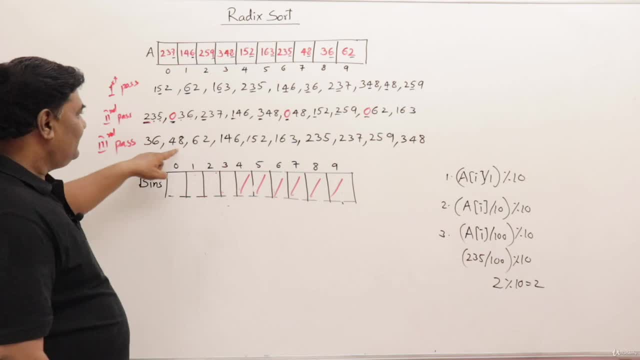 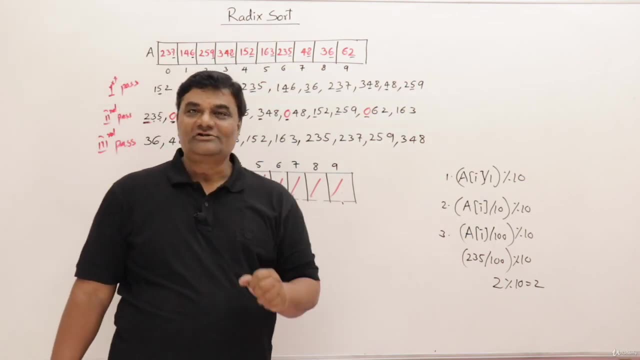 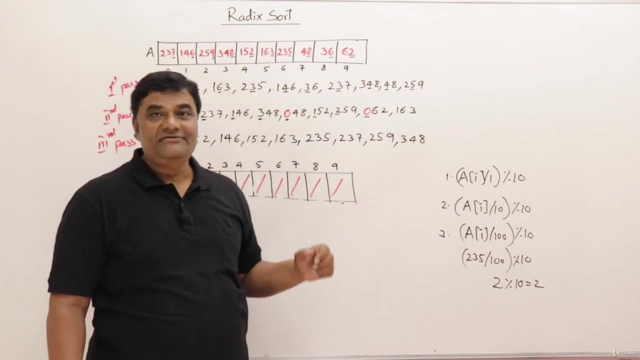 are they sorted? Yes, the elements are sorted. Yes, the elements are sorted. So we have done it in three passes. Say it is similar to count, sort, But the number of passes are more, Because we are not taking bins equal to the maximum element. 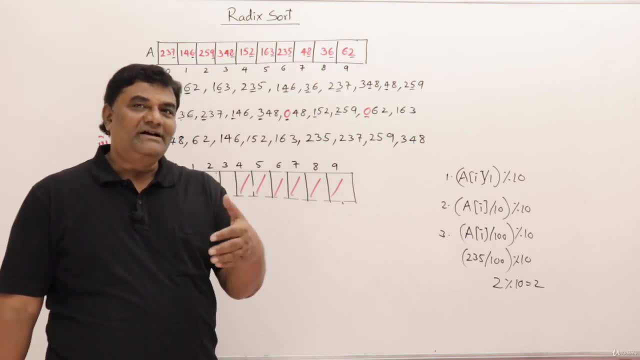 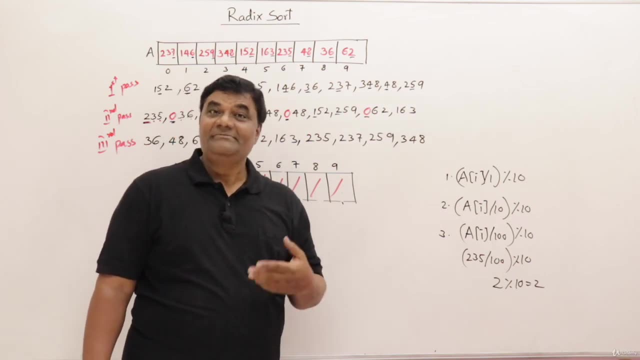 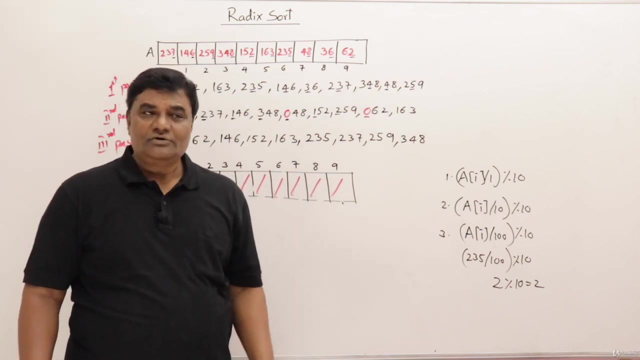 we have limited bins. That is why number of passes has increased. So the time has increased. Yes, time has increased little bit. That is, the process is repeating: Same elements are being done multiple times And that time is depend on number of digits of a number. So 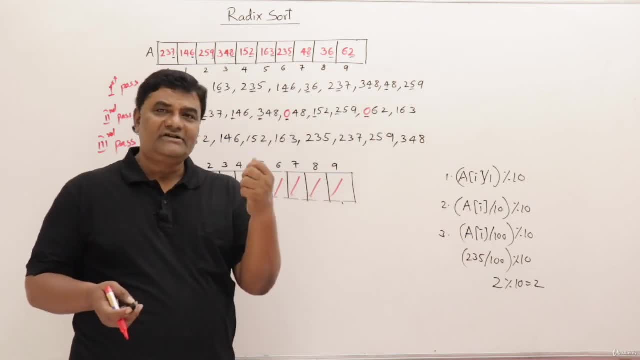 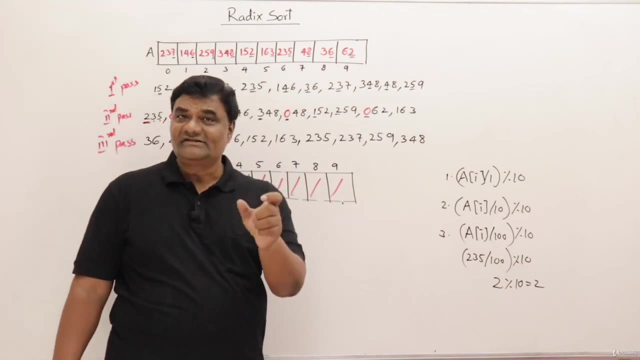 if you have the numbers in less than 1000, then you have to do it three times. Less than 10,000, the second, the third, so everden is having the number of digits and given you have to do it 4 times. So, depending on the largest number that you have, depending on its digits, 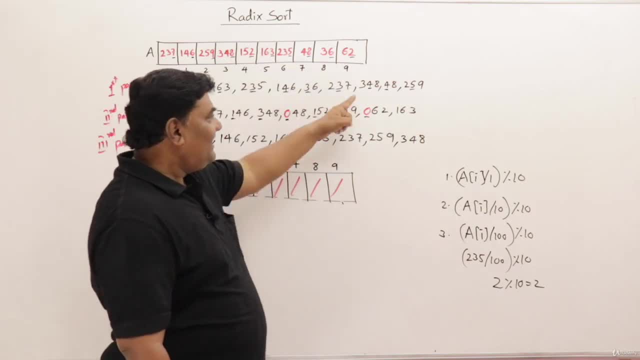 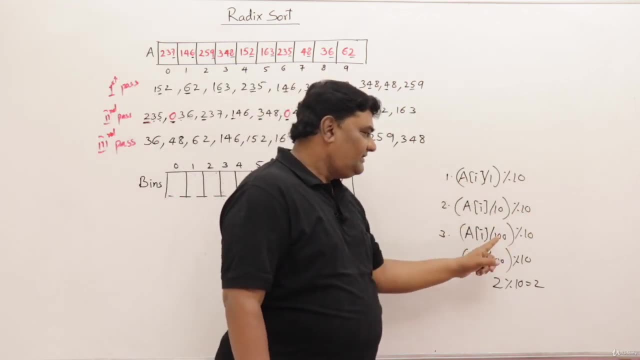 you have to do it that many times And how to get the digits. Lasts the digits, then, second last and the third last from right hand side: Yes, divided by one and more than divided by 10 and more than divided by 100 and more than So, this will give you the digits. So 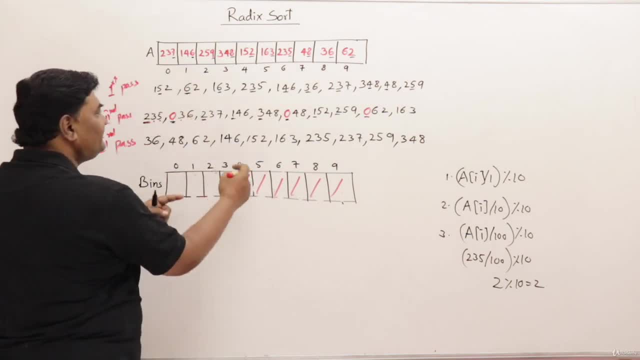 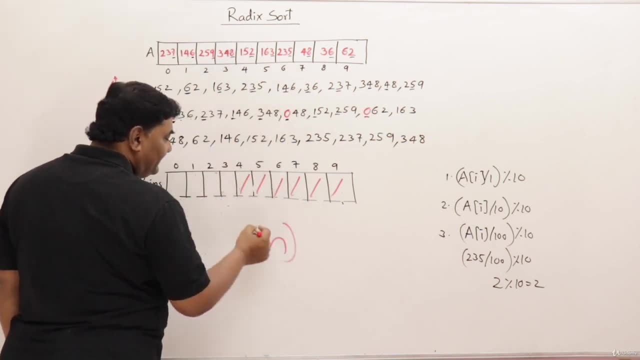 what is the time taken? We are copying all the elements and copying them back there, So it is n, But doing how many times? depending on the number of digits. So, which is wild square? What is until you times, depending on the number of digits. so let us say d into n. now this d is almost like a constant. 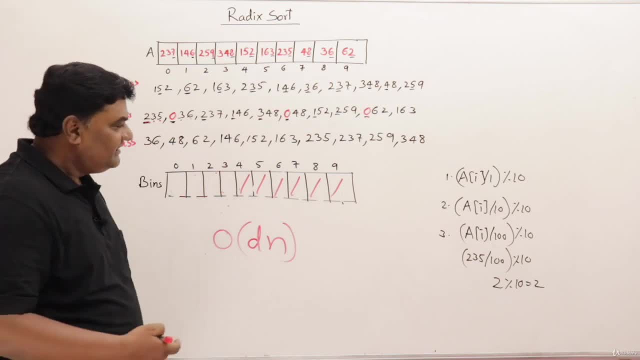 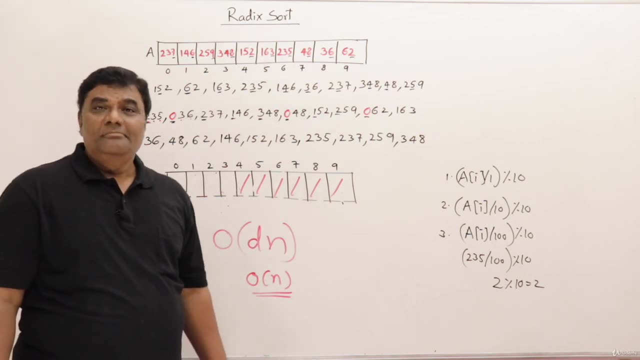 so it's not n times, so it's not n square, so we can say it is order of n, or else say d into n, where d is the maximum number of digits and the space is not not huge, just we have 10 bins and the number 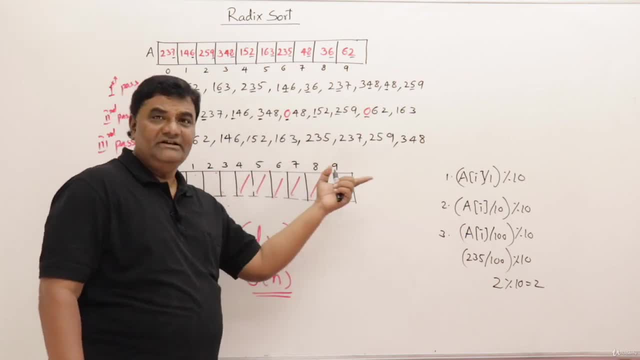 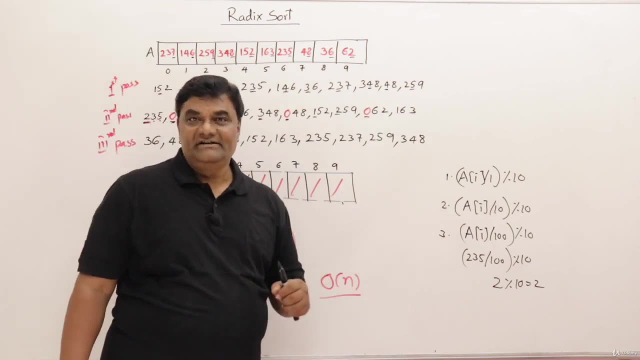 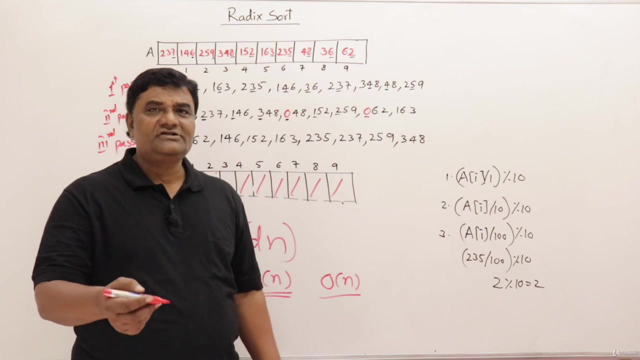 of nodes that will be created in bins depends on the number of elements. so the space is limited and it is n. n means number of bins, so this is limited. it's not a huge space. so that's all about radix sort. the next thing is a function. so that function i will leave it as student exercise. 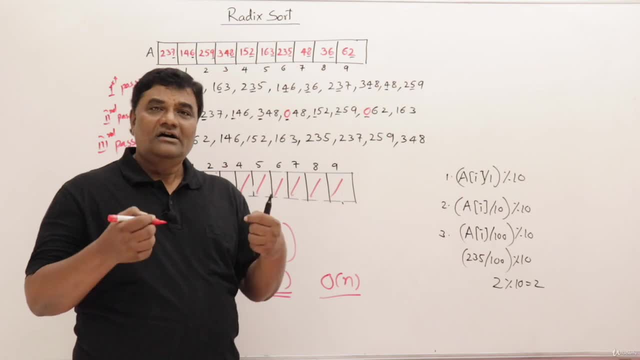 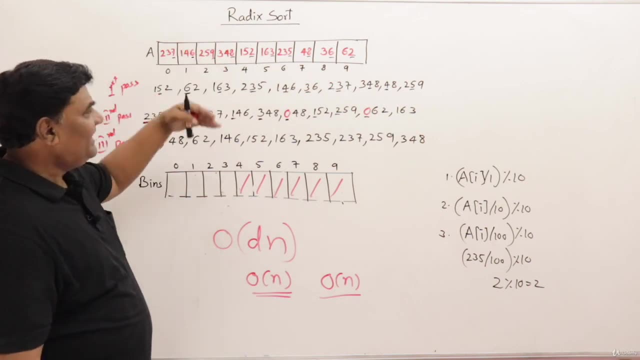 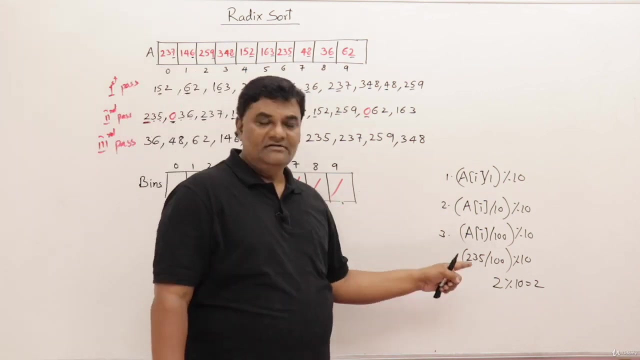 so you write on the function. the function will be almost same as bin sort, only only the thing is the copying of these elements here and again bin sort, only the thing is the copying of these elements here and again bin sort, only back there. this process you have to repeat for some number of times, multiple times. based on this, 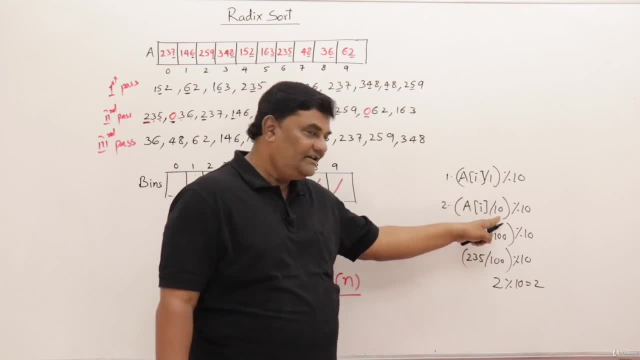 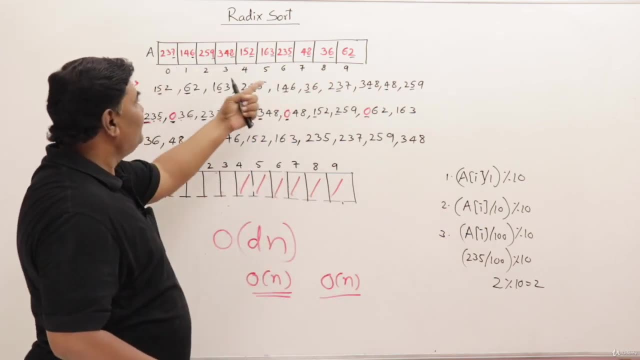 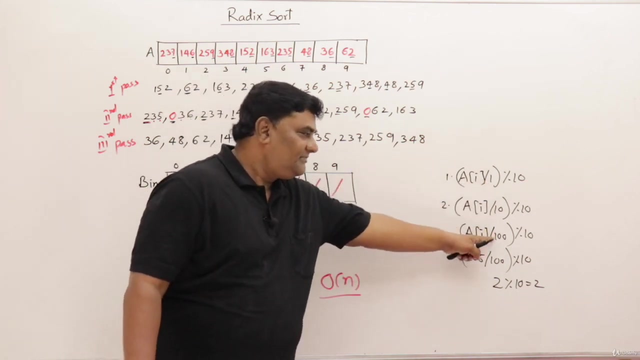 now, this divisor was one. continue divisor was 10. continue divisor was 100. continue: when divisor become next digit, that is, thousand, it is greater than any maximum number. so stop it. so three times you have to run the loop and every time this will be multiplied by 10- 10. so when it is becoming 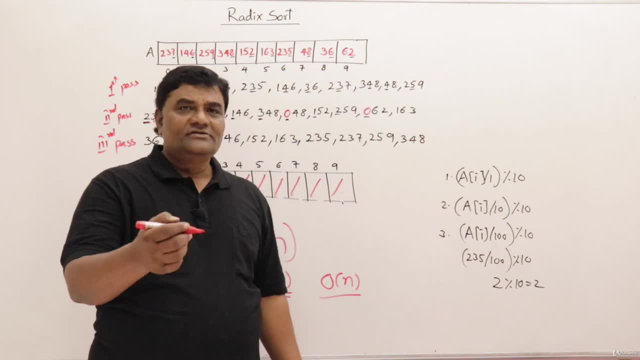 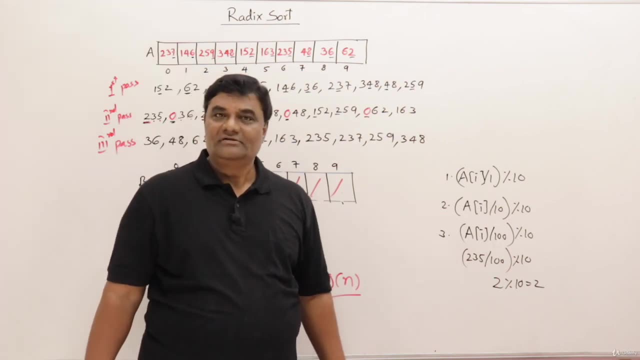 greater than largest number, maximum number- you have to stop. so this is a student exercise. i will not explain it. you have to write down the program and i will be showing you a demo. that's all about radix sort. 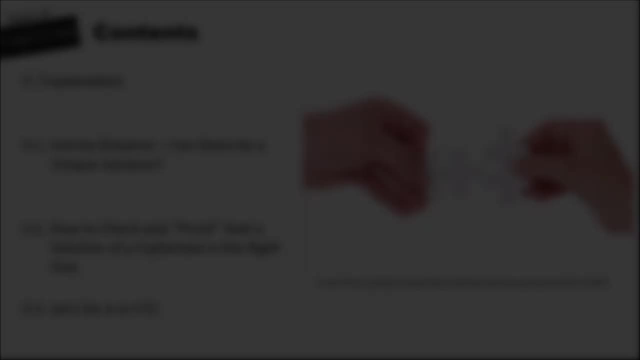 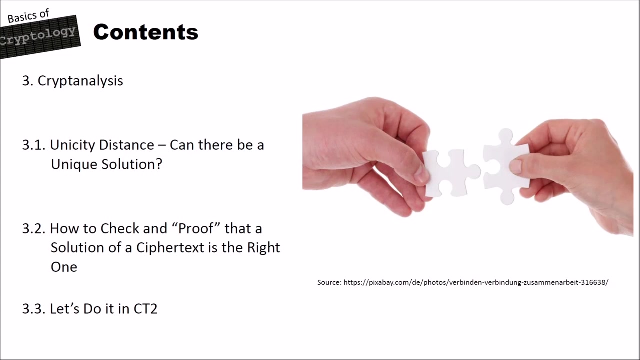 Hello and welcome to a new video on the Cryptography for Everybody channel. In this video in the Basics of Cryptology series, I want to talk about Unicity, Distance and how to check and prove that the solution of a ciphertext is the right one. I structured this video into: